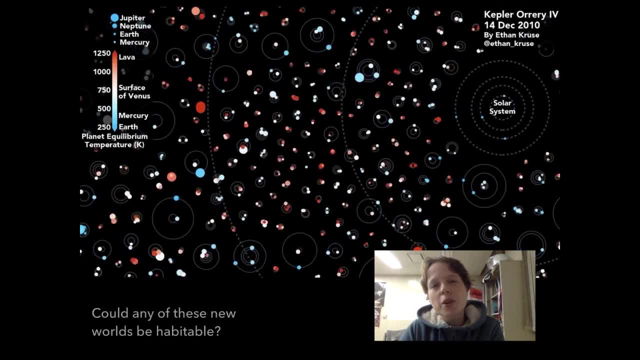 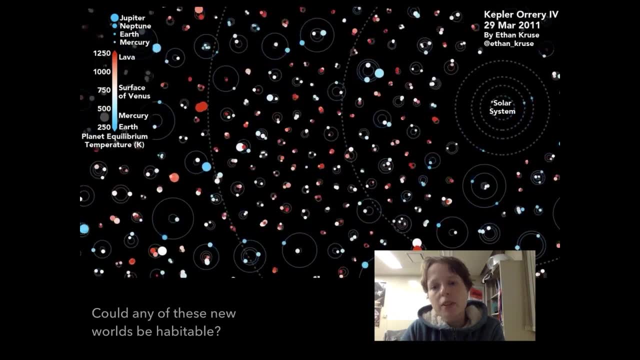 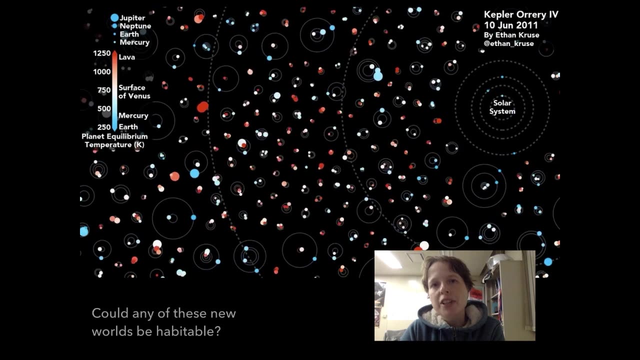 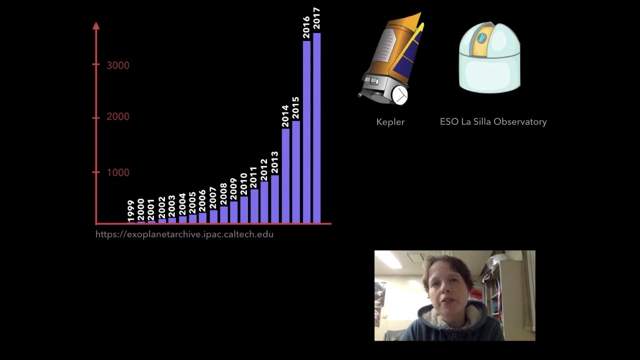 Other than our sun. This results in an obvious question: Could any of these newly discovered worlds be habitable? The problem with that question is, while we have discovered many worlds, we actually know very little about each planet. The majority of planets we have discovered so far have been found by one of two techniques. 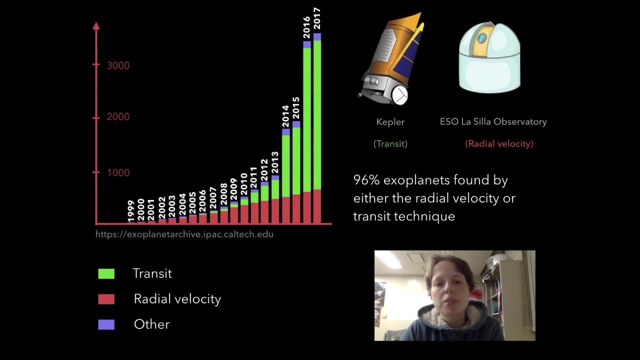 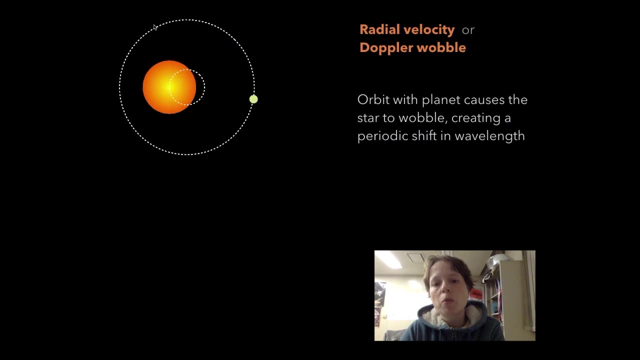 The radial velocity technique used by ground-based telescopes Such as the ESO Observatory in Chile, Or the transit technique used by instruments such as the Kepler Space Telescope and its successor, TESS. The radial velocity technique, sometimes known as the Doppler wobble, detects a planet via the tiny wobble it excites in the star. 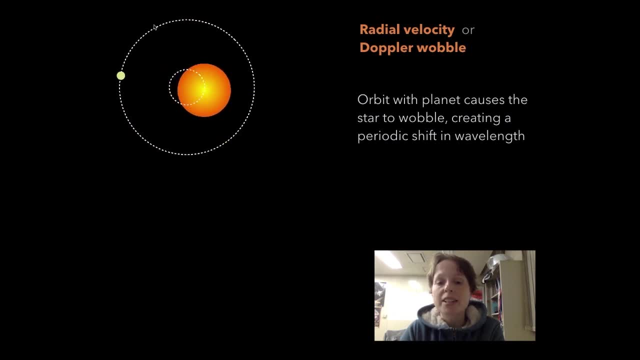 While we normally think of the star as stationary and the planet in orbit, in truth both the star and planet orbit their common centre of mass, As the star is so much bigger than the planet itself. the star is much bigger than the planet itself. 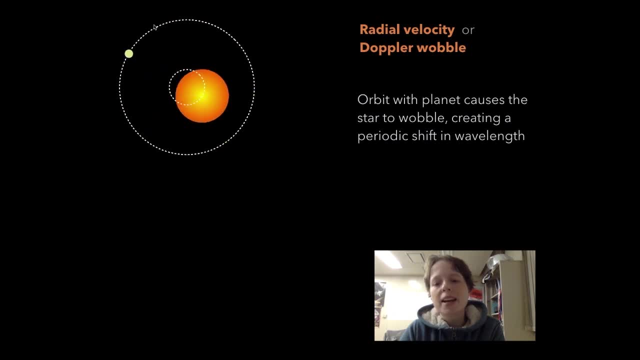 As the star is so much bigger than the planet itself, the star is much bigger than the planet itself. And as the star is so much bigger than the planet itself, the star is much bigger than the planet itself. This centre of mass lies very close to the star's own centre, causing its orbit to be just a tiny wobble in comparison to the planet's wide circuit. 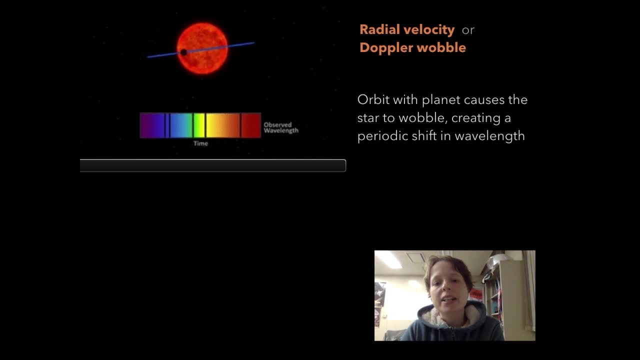 This wobble causes the star to move periodically slightly further away and then closer to the Earth. As the star moves slightly from the Earth, its light waves stretch out and redden slightly. Conversely, as the star moves back towards us, the light waves compress and become bluer. 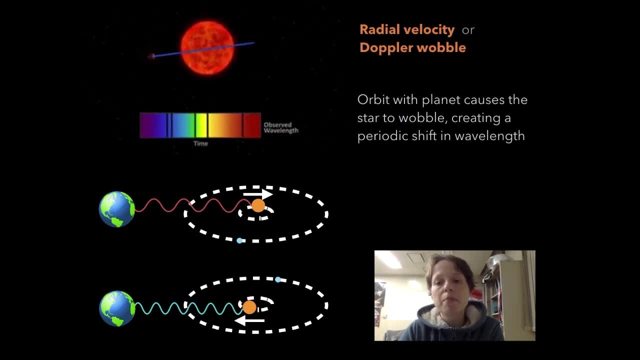 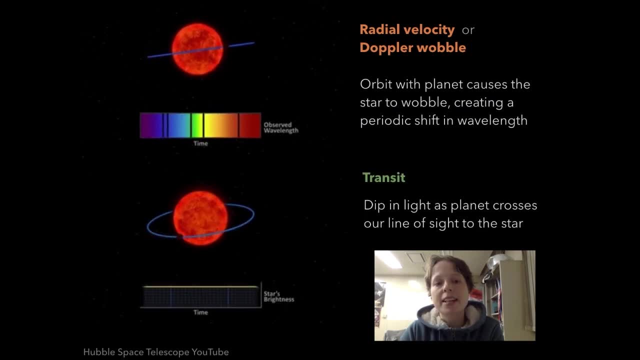 This regular shift from red to blue is what astronomers can measure to detect a planet. The second main method for planet detection is a transit technique. Here, a slight dip in the star's brightness is detected as the planet passes in front of the star. 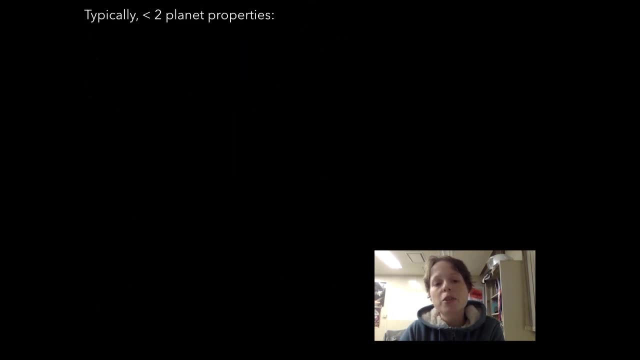 as seen from Earth. These two methods give you just two properties about the planet. The transit technique gives you an estimate of the planet's radius, while the radial velocity technique tells you about the planet's minimum mass. This may be significantly less than the true mass. of the planet, as the radial velocity technique only measures the wobble of the star directly towards the Earth. If the planet's orbit is tilted with respect to us, then part of the star's motion will be directed away from us. We won't measure this and so underestimate the planet. 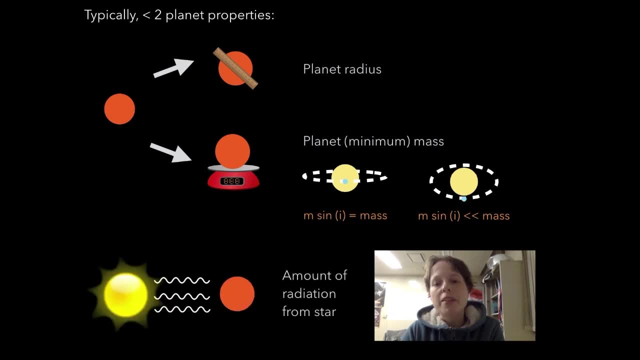 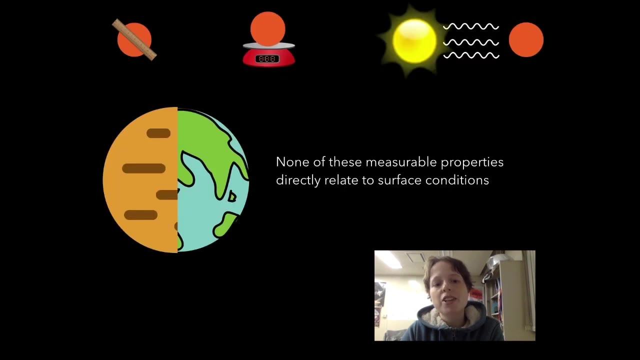 mass. Both techniques also tell you about the amount of radiation the planet receives from the star, but this can be very different from the surface temperature, as it does not allow for the heat-trapping effects of the different atmospheric gases, The challenge we're trying to determine. 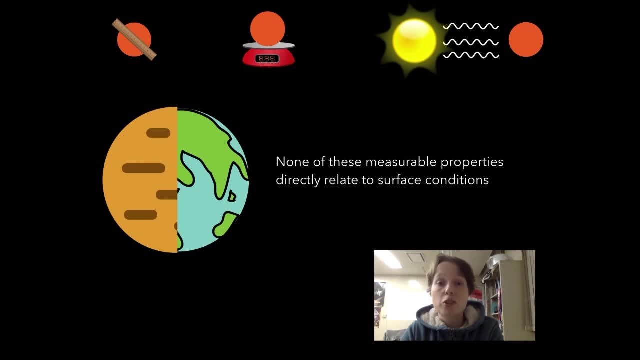 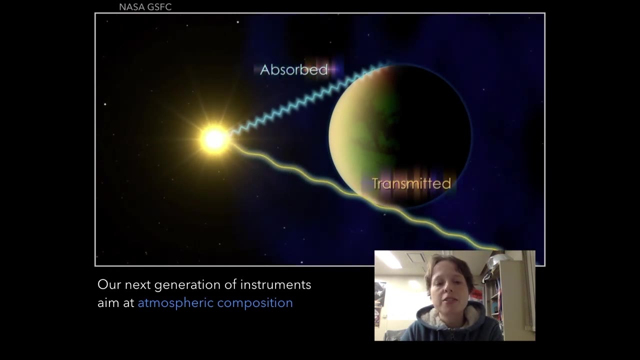 if a planet is habitable is therefore, that we can only measure two or three properties, and none of these actually tell us what it's like on the planet's surface. This will change as the next generation of telescopes will be able to detect light that passes through the planet's 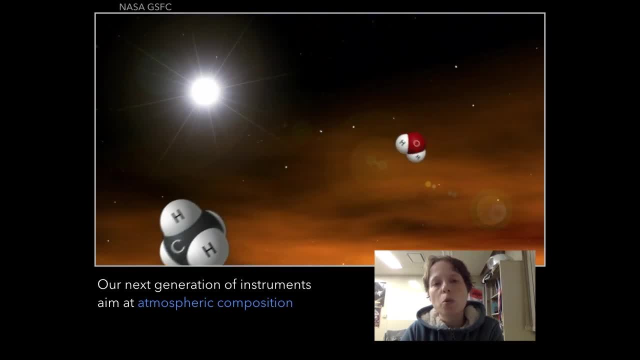 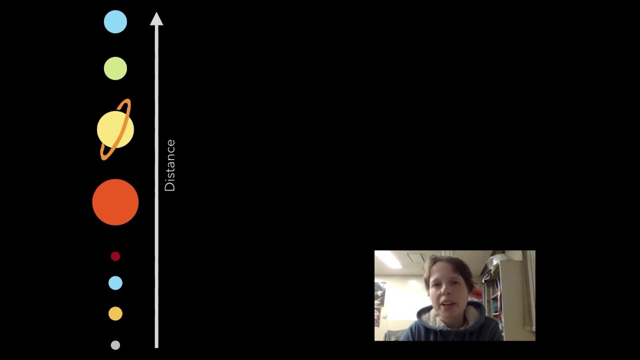 atmosphere. Different molecules in the atmosphere absorb different wavelengths of light, providing a fingerprint of missing wavelengths that indicate atmospheric composition, our first hint of what is happening on the planet's surface. But this brings us to a new problem: Such atmospheric spectroscopy for rocky, temperate planets. 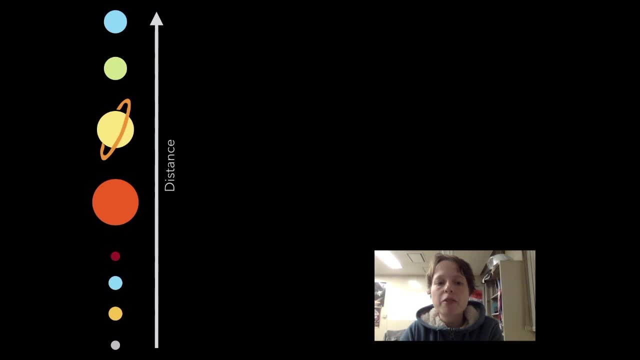 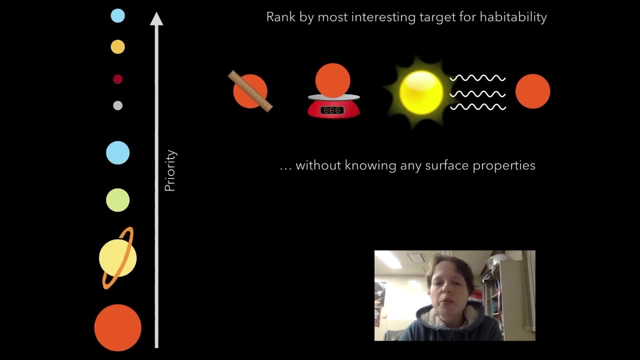 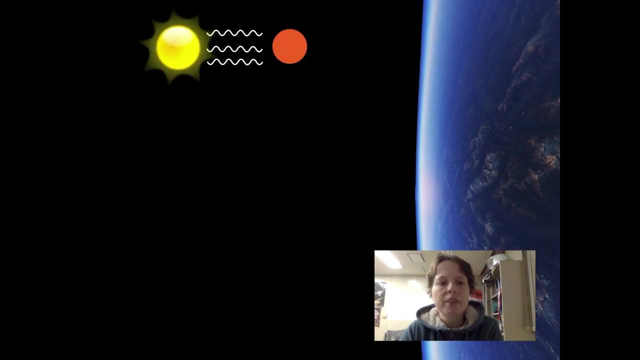 is time-consuming and difficult. We therefore need a way of selecting planets most likely to reveal interesting results. But how do we select planets best suited for habitability without knowing any surface properties? Let's think about what we want to find. It's going to be easiest to recognize Earth-like life. 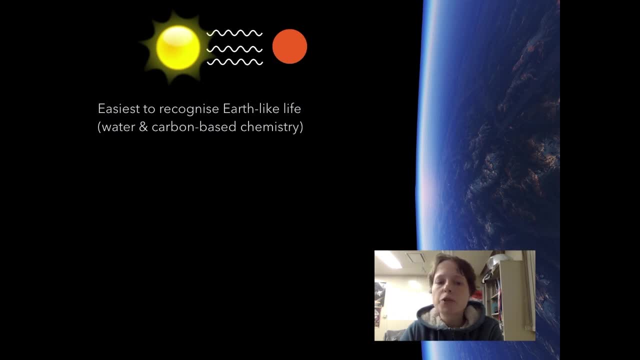 that is water and carbon-based chemistry. Also, this needs to be detectable, which means that we need water on the surface of the planet, not a subsurface system like Europa. Based on this, we can ask the question: how much insulation does an Earth-like planet need? 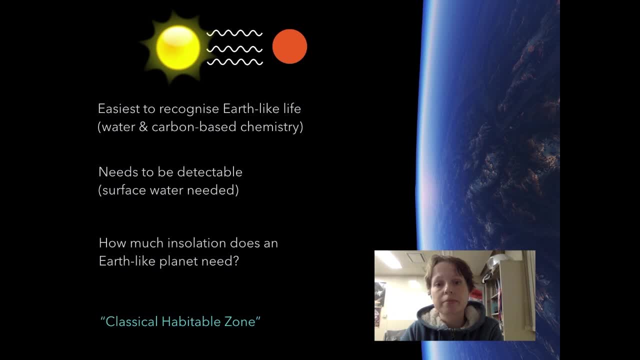 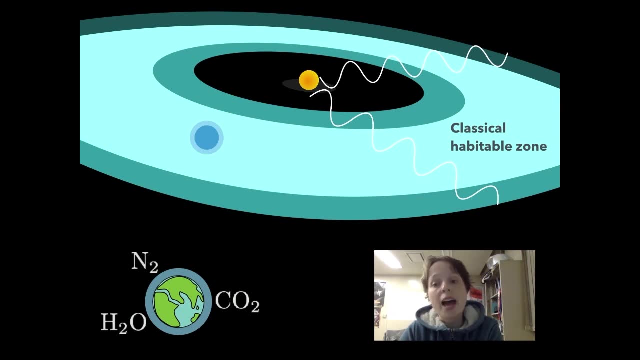 The answer to this is a classical habitable zone. The classical habitable zone is where an Earth-like planet, that is, a planet with our surface pressure, atmospheric gases and geological processes can support water on the surface. Often in exoplanet literature, this is simply referred to as the habitable zone. 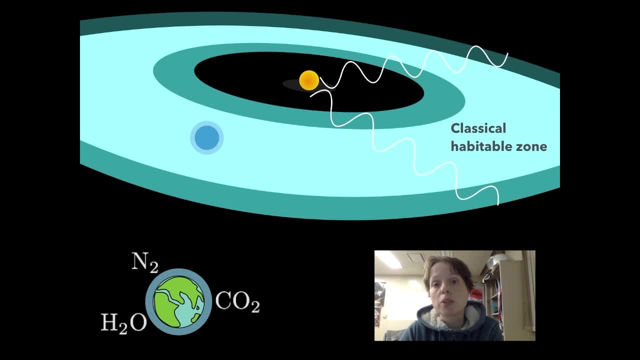 as we don't yet know about planets other than the Earth that can support life. At the inner edge of the habitable zone, it is too warm for surface water on the Earth and it evaporates. At the outer edge, carbon dioxide condenses into clouds. 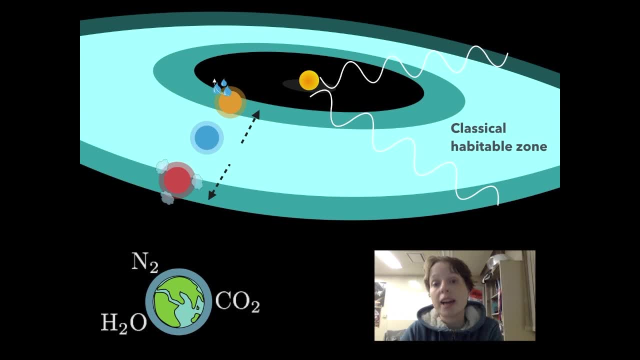 and is no longer able to provide the thermal insulation of a greenhouse gas, so the planet freezes. Climate models predict that the habitable zone can support life. Climate models predict that the habitable zone can support life. Climate models predict that the habitable zone can support life. The habitable zone should stretch between 0.99 AU and 1.67 AU, where 1 AU is the average distance of the Earth from the Sun. Our planet therefore sits right on the inner edge. A slight extension to this is known as the optimistic habitable zone. 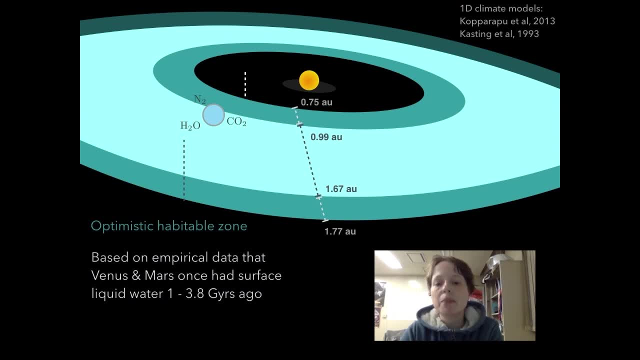 which can broaden these limits based on the idea that Venus and Mars probably have supported surface water in their past. So an Earth-like planet could have a period of habitability just outside the habitable zone edge of the Earth. So an Earth-like planet could have a period of habitability just outside the habitable zone edge of the Earth. 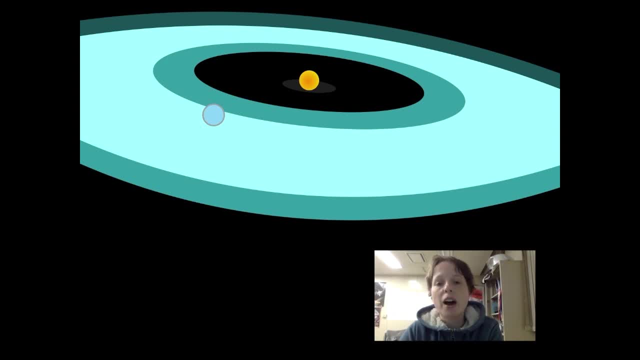 So an Earth-like planet could have a period of habitability just outside the habitable zone edge of the Earth. The edges of the classical habitable zone are only calculated for the Earth. This is easily demonstrated as, while Venus sits outside the habitable zone, 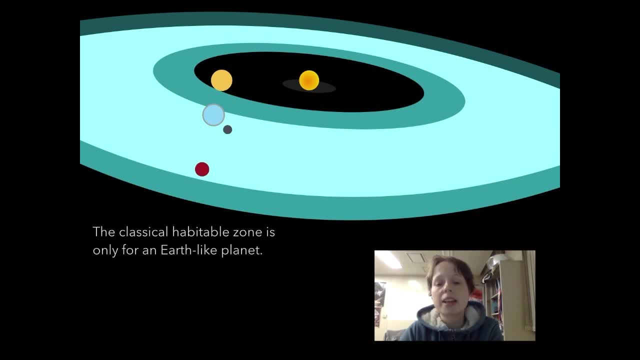 both the Moon and Mars orbit within it, but neither are Earth-like enough to support liquid water in this region. Different planets might have different habitable zones at different locations, or they may not have a habitable zone at all Of the planets we found so far. 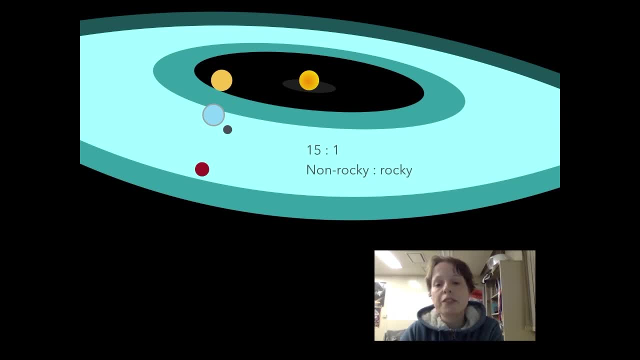 far, orbiting in the classical habitable zone. almost 15 times as many are large enough to likely have thick Neptune-like atmospheres, compared to planets that might be rocky, We have discovered planets that are the right size to be rocky and orbit entirely within the 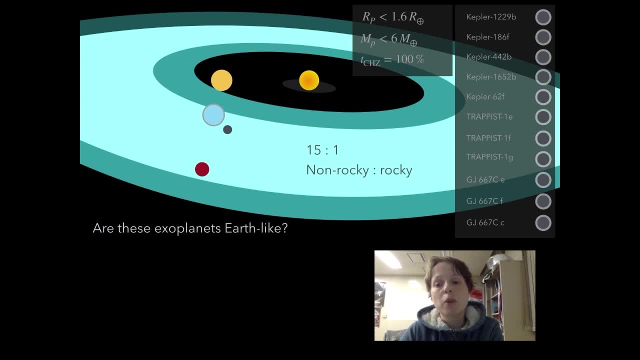 habitable zone. Are these Earth-like enough to support liquid water in this region? We don't know. They may have very different atmospheric gases or geology that makes surface water impossible. The only thing we can say is that if another habitable Earth-like planet is out there, 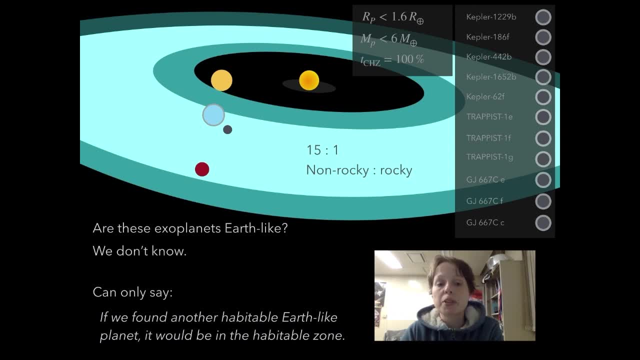 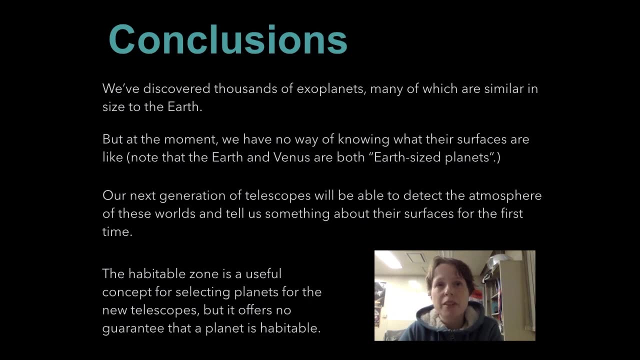 it would be in the habitable zone. But being in the habitable zone does not mean you're Earth-like enough for life. So, in conclusion, we've discovered thousands of exoplanets, many of which are similar in size to the Earth, But at the moment we have no way of knowing what their surfaces are like. 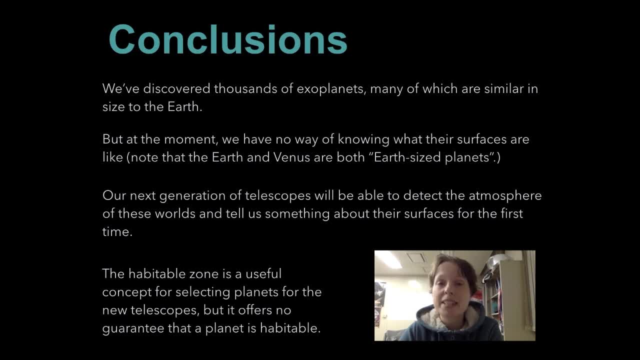 Note in particular that the Earth and Venus are both very similar in size, so they are both Earth-sized planets. Our next generation of telescopes will be able to detect the atmosphere of these worlds and tell us something about their surfaces for the first time. The habitable zone is a useful concept for selecting planets for.